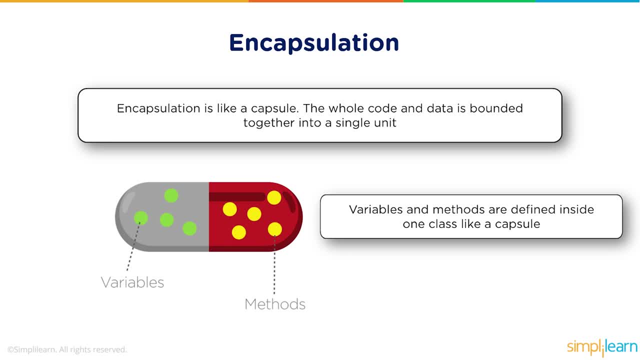 this shield. As you can see, variables and methods are defined inside one class, like a capsule. Now the question is: why do we need encapsulation? The main reasons are: first, better control of class attributes and methods. Second, class attributes can. 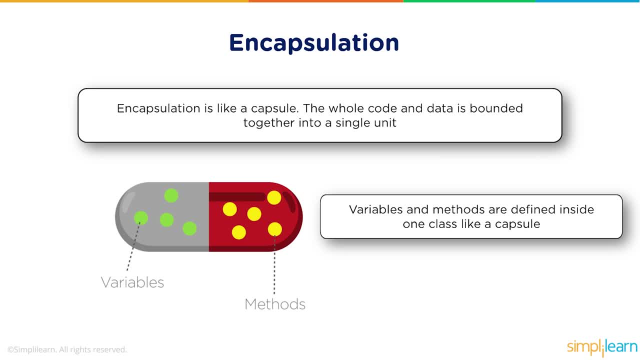 be made read-only or write-only. Third, it makes Java code very flexible. This means the programmer can change one part of the code without affecting other parts. Apart from these, encapsulation is mainly used to protect data and increase security of the code. As you can see, to protect the. 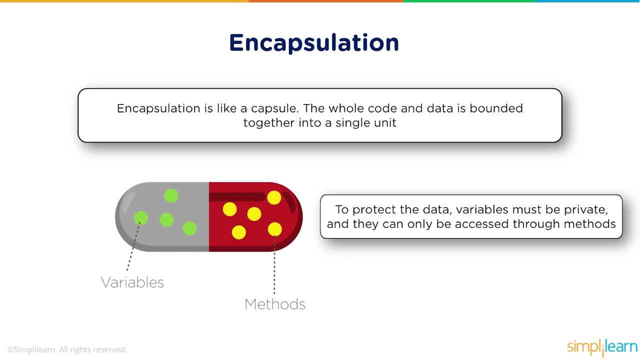 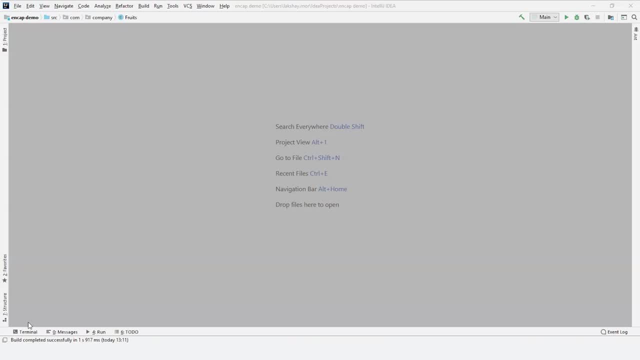 data variables must be private and they can only be accessed through methods. Now let's see Java code for encapsulation to understand the concept better. So now let's create a new project. First, we are going to create a new class. 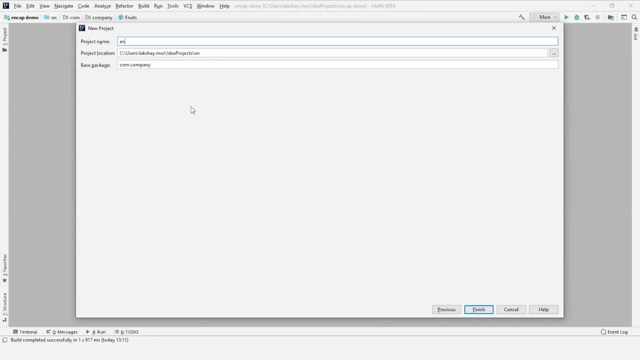 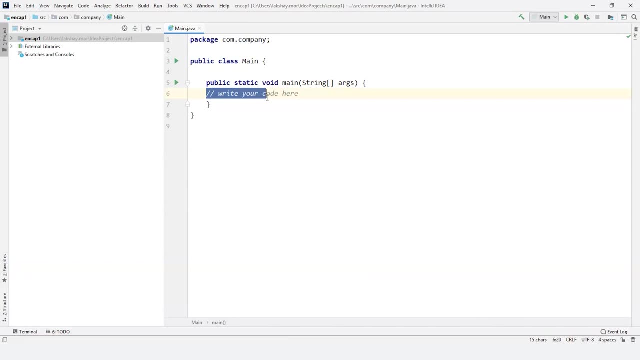 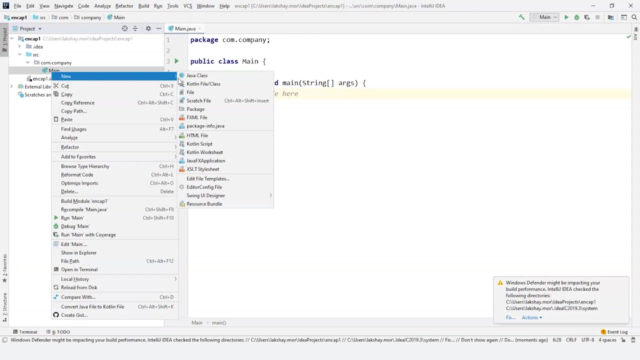 Next, next, and I'm going to name it as ncap1.. So here we have our main class. We can write the code here. So, before writing the code, let me create a new class. Right click new Java class, And I'm going to name it as employee. 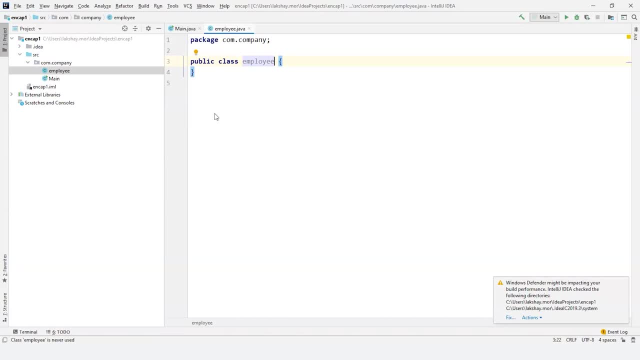 So in this program we are going to use a classic example of employee Using employee name, id and salary. So in this class let me create variables: First string name, then integer id and then int salary, So I can easily use these variables. 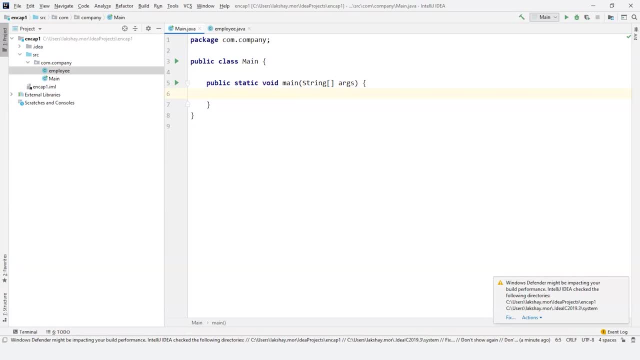 in our main program by creating object of the class. So let me just create the object employee. Now I can use eid name or salary, anything I need to, But this program is about encapsulation. So this is an easy program we can do. But in order to secure our programs when we have 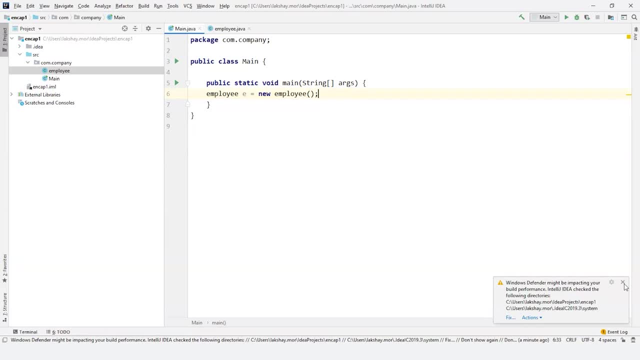 a large number of program and large number of lines in a program. So we need encapsulation at that time so that data can be secured. So for that I'm going to name it as private. Now all three variables are private, So I can't use them. See, we can't see them anymore. 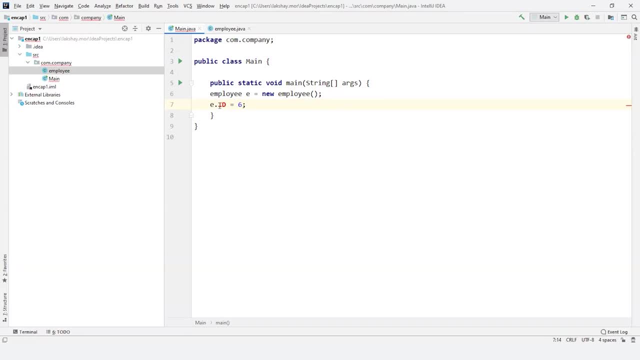 If I write id, we'll get a red color here. So if we go on it, we can see id has private access. So that means we can't use it directly. Because of this, we need getters and setters. that are normally methods that are used for these. 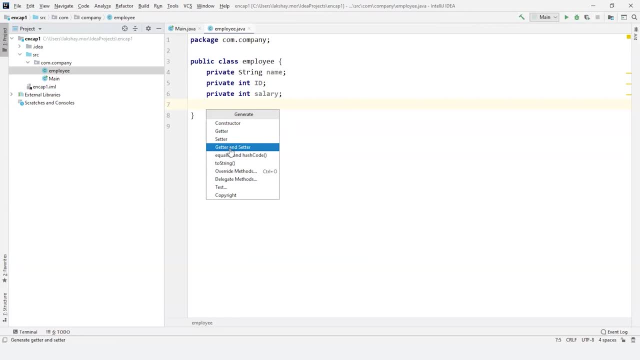 So right click generate And we can see that we have a private access. So we can see that we have a private access. So that means we can't use it directly. Because of this we need generate. But here you can see getters and setters, So just select all. 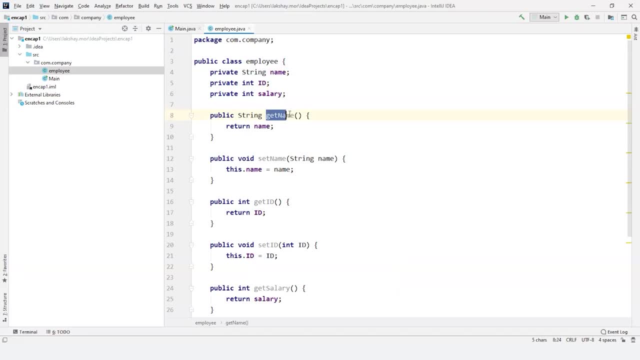 of them And okay, So now we can use these methods instead of directly using the variables, So we can get in the starting, Then set, Then get And again set. So likewise it goes like this: So now we have set here. So if I want to, 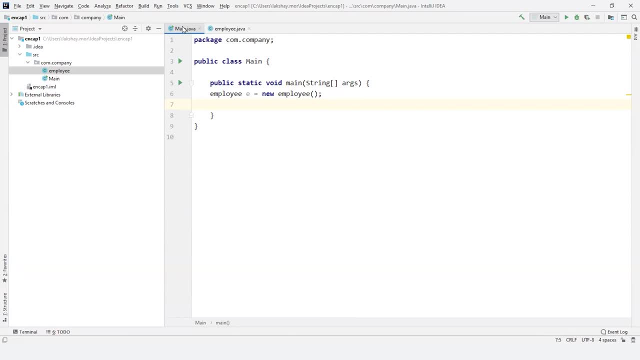 declare variable and if I want to put some value inside my variable, so how can I do that? So here you can see getter, getter, getter, And again we can see that we have a separate stage setter and answer. So now, if we set, 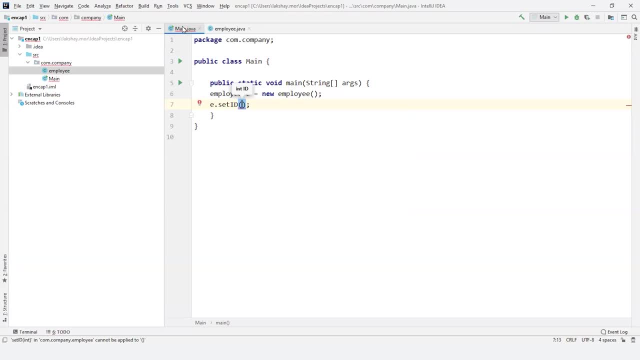 ID or get salary. so if I go for get ID- sorry, if I go for e- dot set ID and I set it as 6, so this shows no error. this means we can use methods to access variables. so let's complete our program now. first I'm gonna set everything. 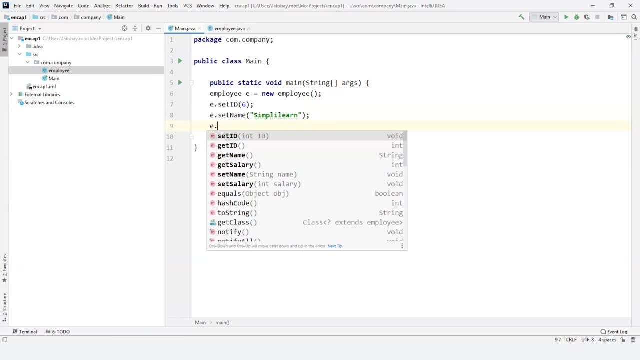 and lastly, e dot set salary. let's get it as 30 thousand, maybe in dollars or maybe in rupees. let's just set it as 30,000 for now. so how I'm going to print it for this, I'm going to go to a print statement and then name: 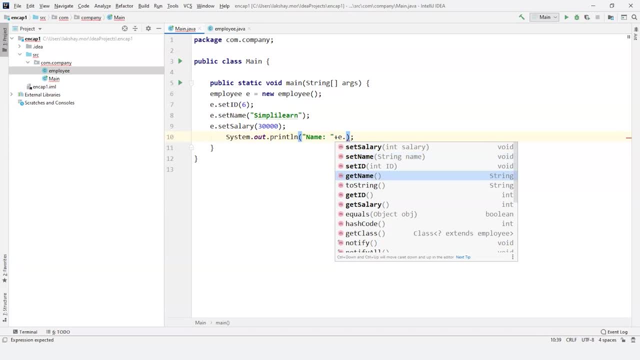 and e- dot not set name. but this time I'm going to go with get name. get name is to return the value of e- dot set name and e dot dot set time I'm going to go with get name and e- dot not set name. but this time I'm going to go with get name, get 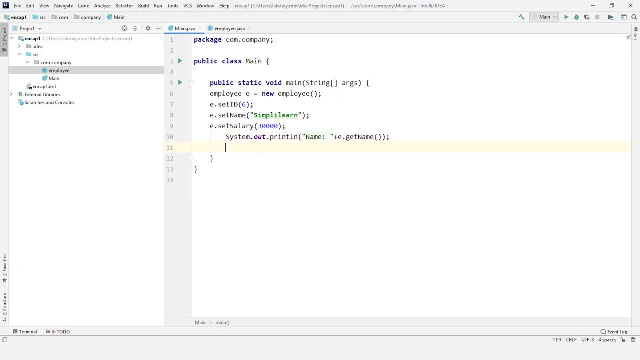 of the name that i have given. so in this case, that simply learn. and next will be id, and e dot get id. and lastly, salary- e dot get salary. so this is a simple program that is used to define encapsulation. if we don't use private variables, that becomes a normal program. 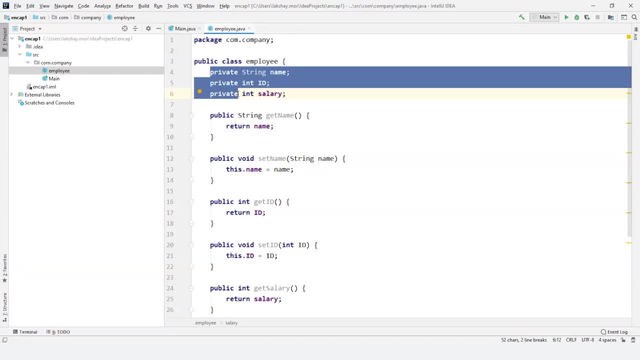 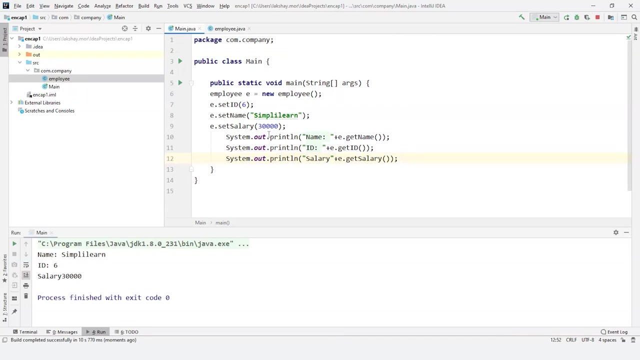 so when we use encapsulation, we are going to use private every time whenever we declare variables, so that it's secure and no one can access the variables directly. so now let's run the program and there we go. we have our result. we have executed the program successfully. 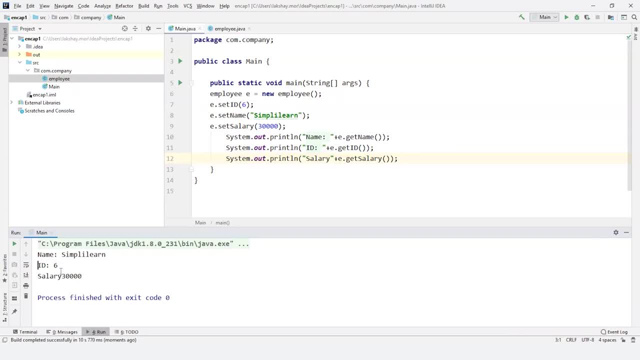 and as you can see name, simply learn id 6 and salary is 30 000. so i hope you understood the concept of encapsulation. so the main concept of encapsulation is: all the variables can be accessed through methods, so for this we use getters and setters. 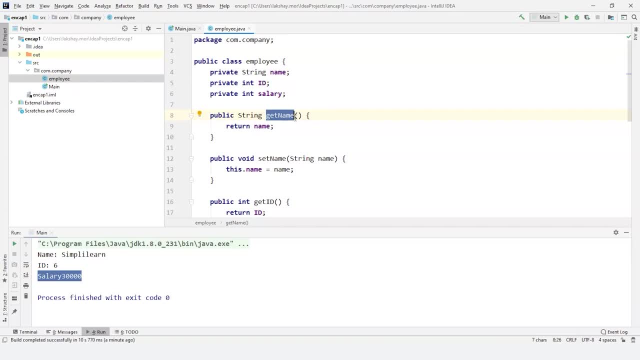 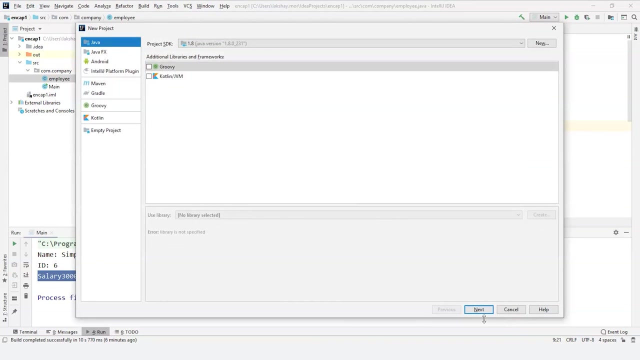 that are inbuilt functions for intellij or netbeans or eclipse. so with this let's move on to our next program, to understand it better and how we can manipulate these variables or methods using program. so again, let's create a new project, and this time i'm going to name it as encapsulation. 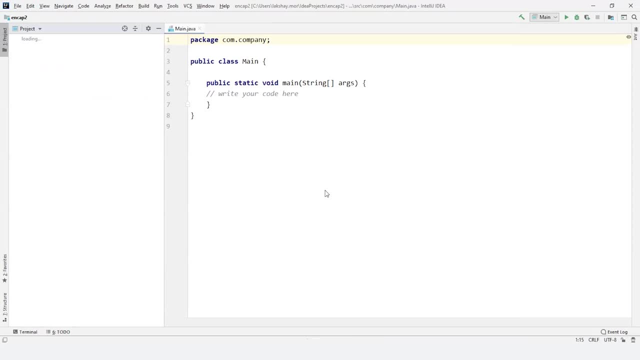 2, because it's the second program for encapsulation, and here we have our main program now. this time i'm going to use an example of cars, so let me just create a new class and i'm going to name it as cars. so in this again i'm going to create three variables that are private. 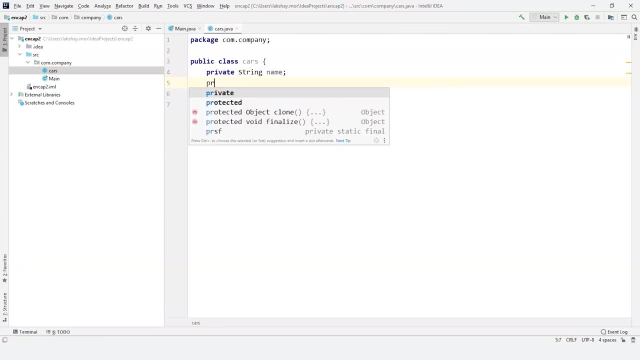 so first i'm gonna get string name, then private string price means price of the car and third one top speed of the car. so we can create the program that we did before as it is, but i'm gonna explain you more in depth how we can manipulate these variables or classes. so i'm gonna create a constructor for the class. 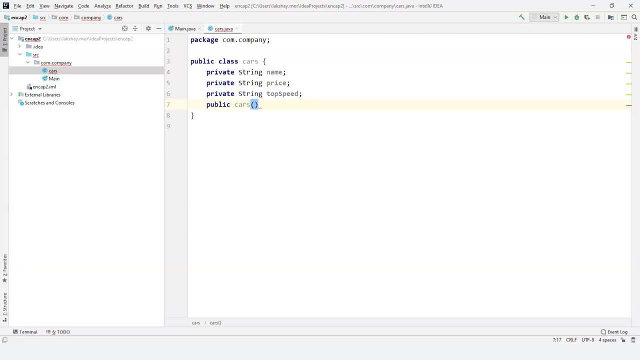 cars and inside. i'm gonna give it as arguments as string name, then string price and string top speed and i'm gonna give it as this dot name is equal to name. this is so that the class can identify that we are going to give arguments related to that and the class can return the values of it. 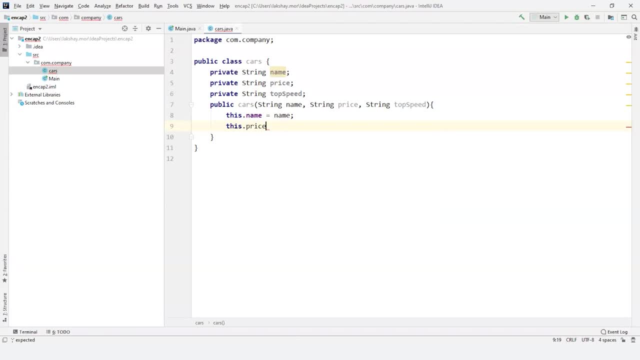 so similarly, i'm going to give it, as this dot price is equal to price and, lastly, this top speed is equal to top speed. so with this we have completed our constructor for it. now let's have getters and setters for the same thing for these three variables. so generate getter and setter, select all and okay. 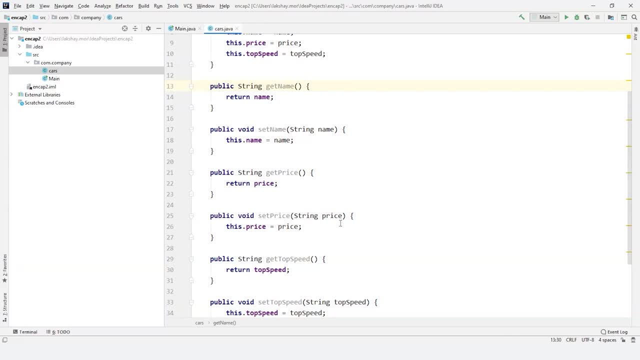 this is a great feature that we have in java: getters and setters. otherwise we'll have to type the whole code. so with this let's move on to our main program. we'll write the code here. first i'll create object of the class cars and inside this i'm gonna give arguments, or inside this i'm gonna give values that i use in. 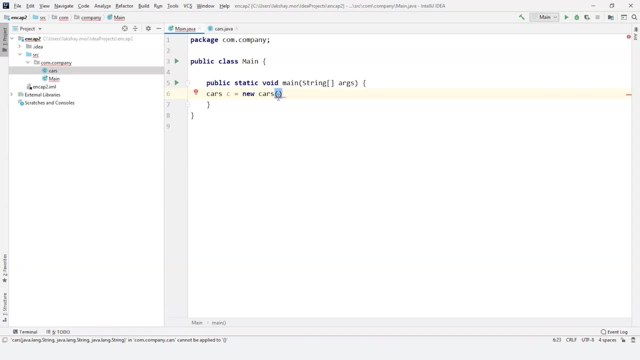 constructor to assign the values without using any c dot get name or c dot get price. so my first was name, so let me just name it as bmw. the second thing was price, so i'm gonna give it as thirty thousand dollars. and the third one was top speed. so top speed, i'm gonna give it as two hundred kilometer per hour. 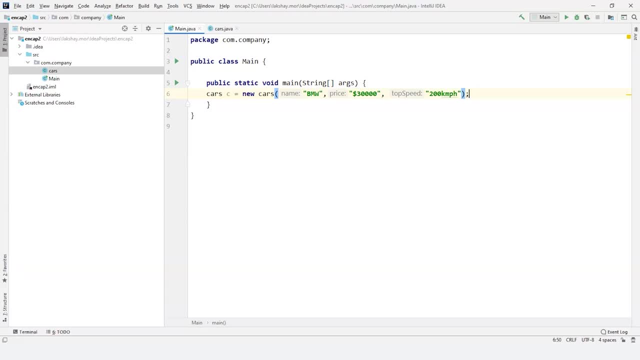 so we have assigned all the values to the variables and we have created object as well, all in the same line. so this is another way of creating objects, or another way of assigning values to the variables that are private. so if i try to print these, they can be easily printed. 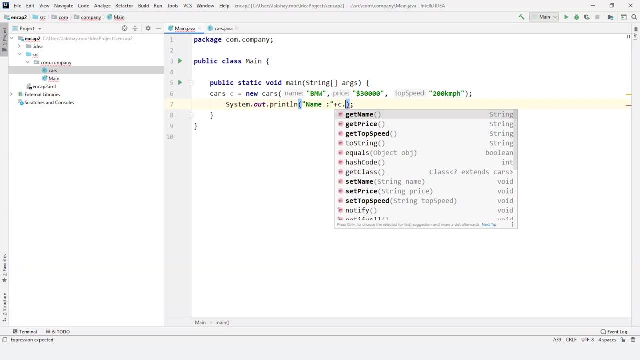 so in the starting name and c dot. so this time i'm gonna give get name so it automatically gets the value that i assigned to the variables through getters and setters. after that price, price- c dot. price get price and in the end top speed- c dot, get top speed. so if i print this, let's execute it. 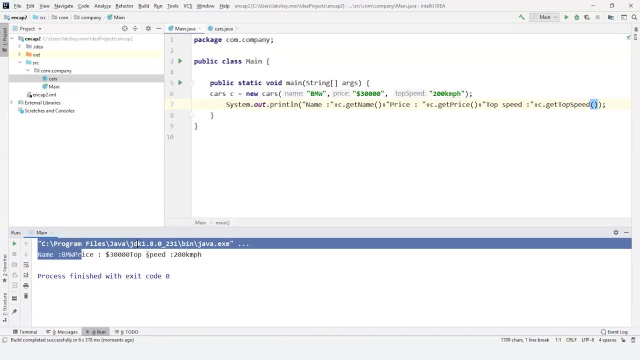 and there we go. we have name bmw, price and even the top speed. now, if i give spaces between them, it will look neatly, so let me execute it once more. and here you go: name bmw, price: thirty thousand dollars and top speed: two hundred kilometer per hour.